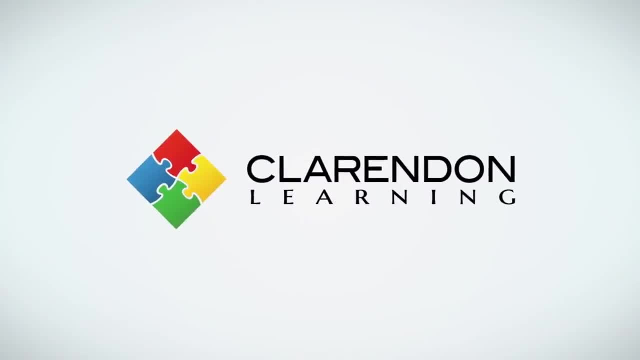 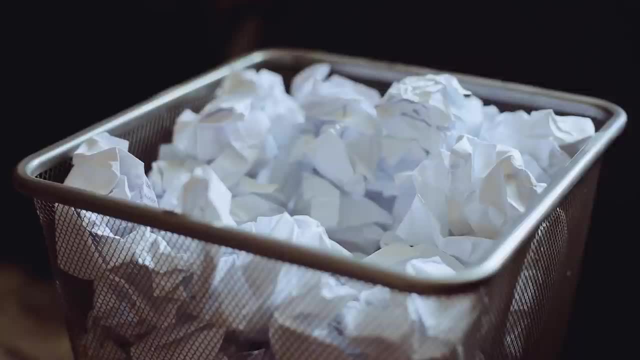 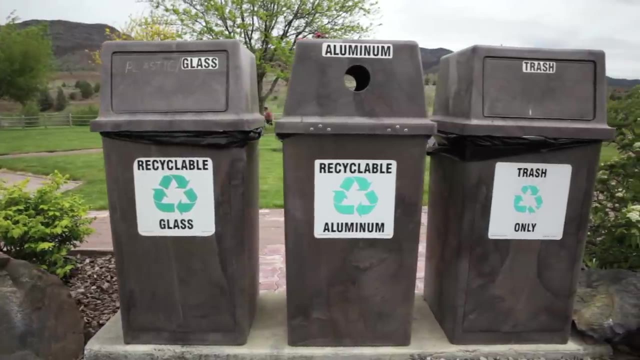 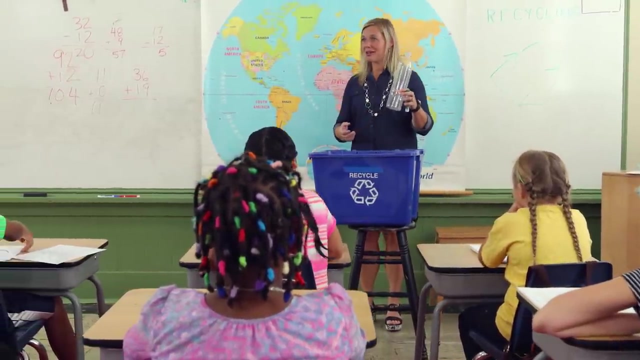 Recycling for kids. Do you have a special bin box in your classroom where you place your used papers? Have you ever seen garbage cans in restaurants and on the street that say recycle. At home or at school you may be encouraged to recycle things like bottles, paper and other. 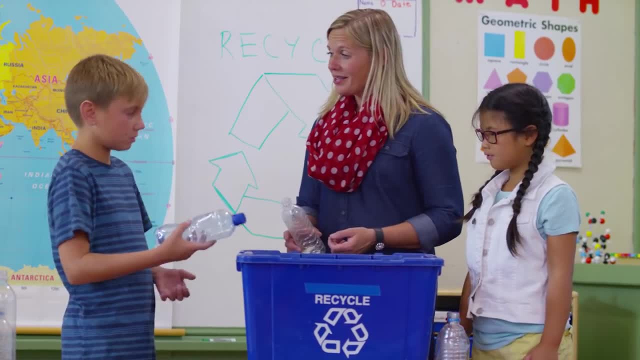 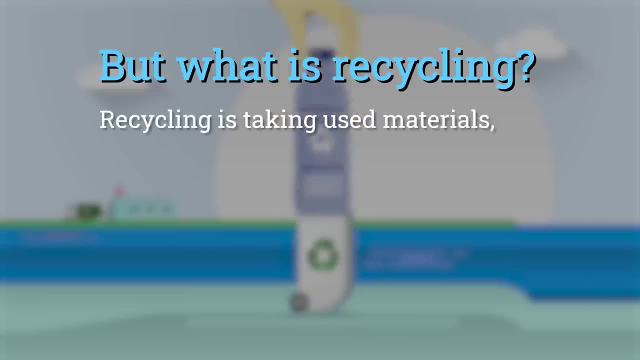 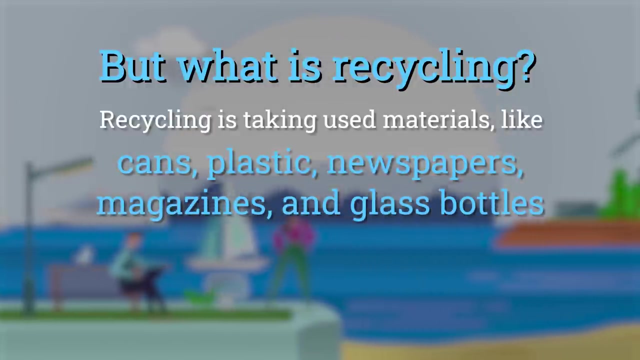 items when you're finished with them, instead of just throwing them into the trash. But what is recycling? Recycling is taking used materials like cans, plastics, newspapers, magazines and glass bottles and turning them into new products that we can use again. 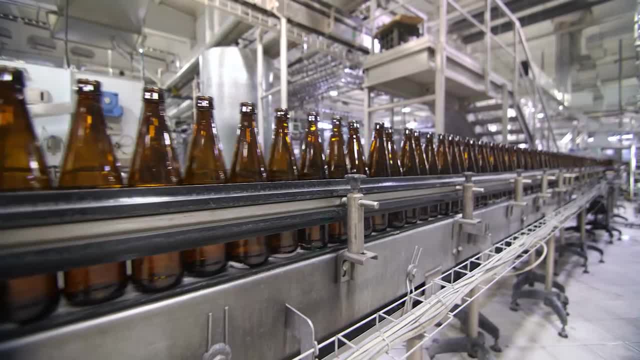 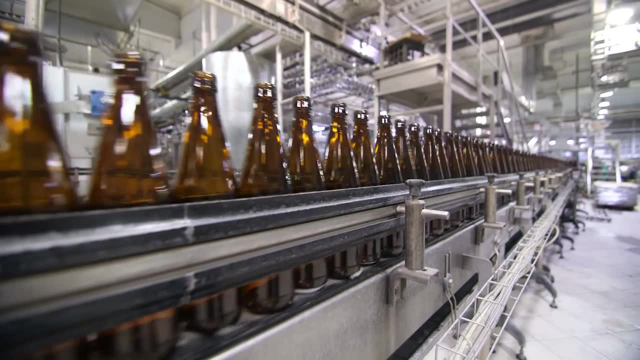 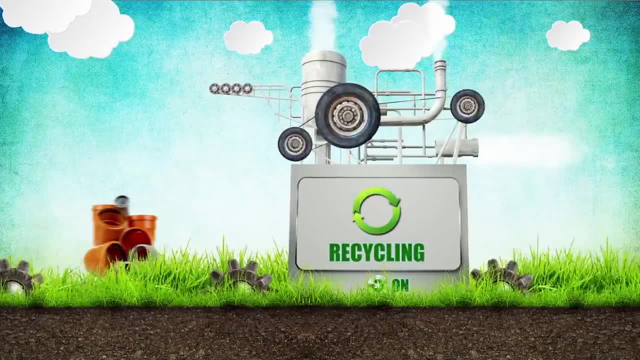 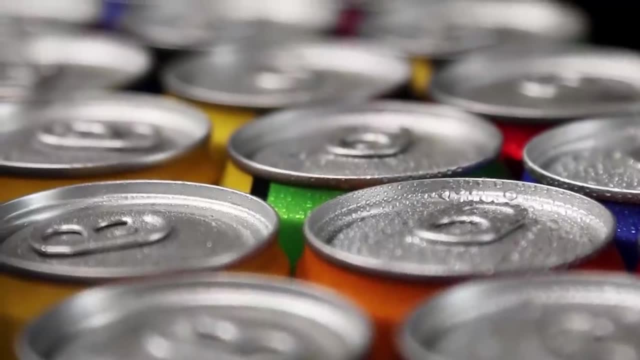 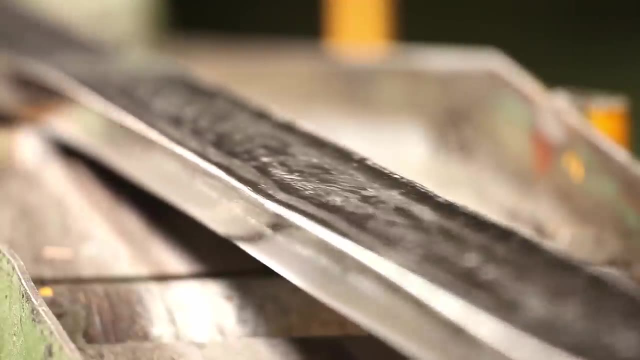 ways, depending on what the item is. For example, magnets are used to separate different types of cans, and then they are washed and smashed. After that, the cans are melted down in a hot furnace, and then the metal is formed into something new. Paper, on the other hand, is chopped into tiny 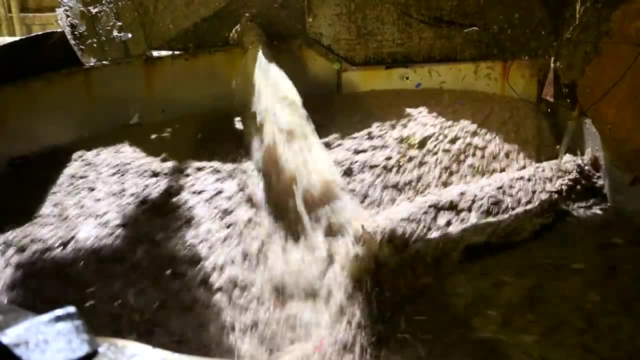 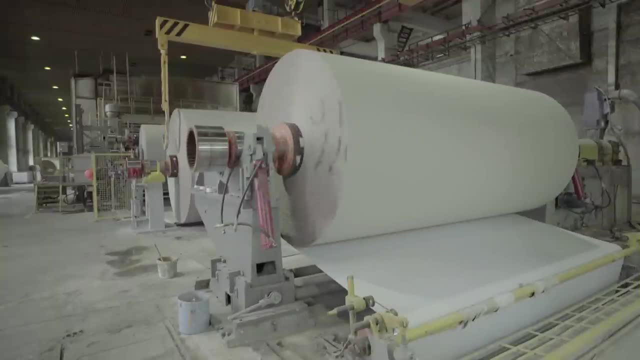 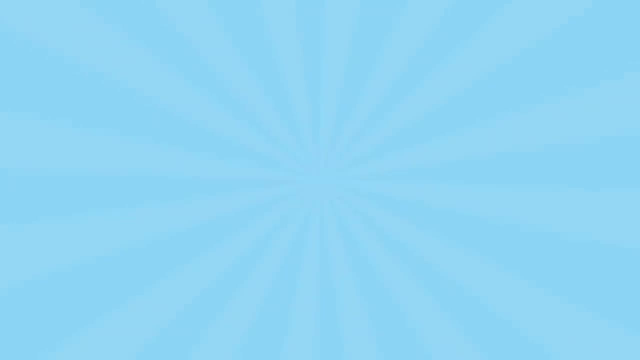 pieces then turned into a pulp by adding water. After that it's bleached and chemicals are added. Then it's ready to be made into new paper. Pretty neat, huh. One of the goals of recycling is to reduce waste. When you think about the ways you can help cut down on waste, 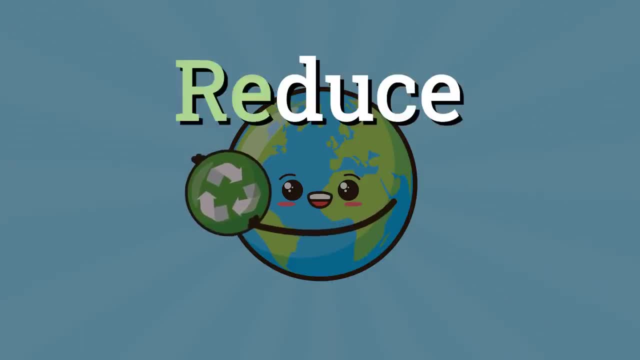 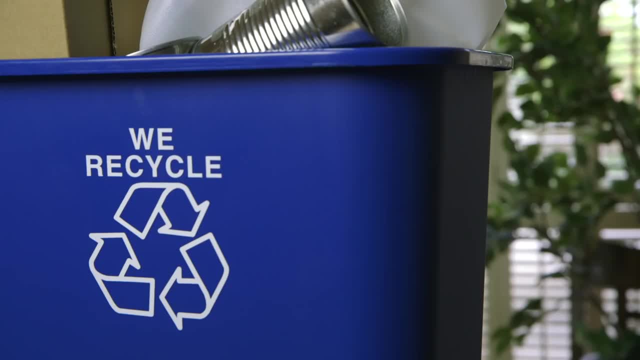 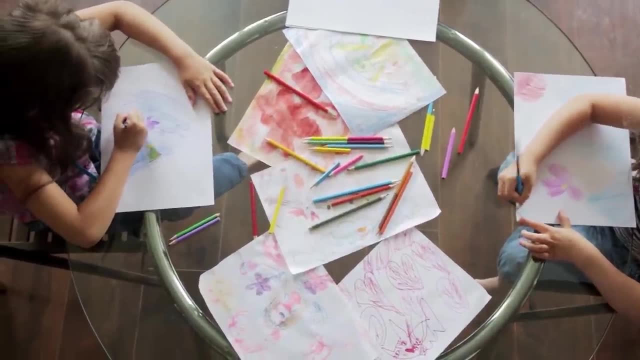 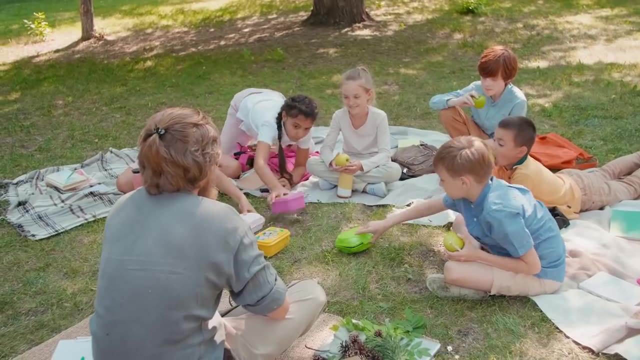 recycling. But what about the other two R's? To reduce simply means to cut back on the amount of trash you make. Instead of getting a new piece of paper every time you want to draw a picture, try using the back of an old piece of paper If you bring home lunch to school. 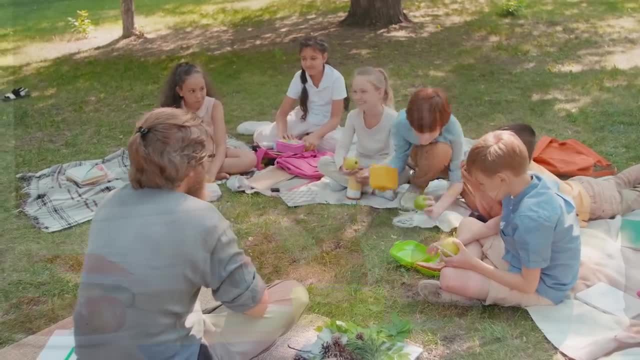 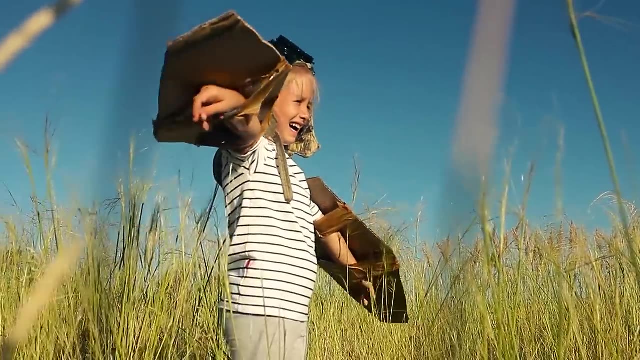 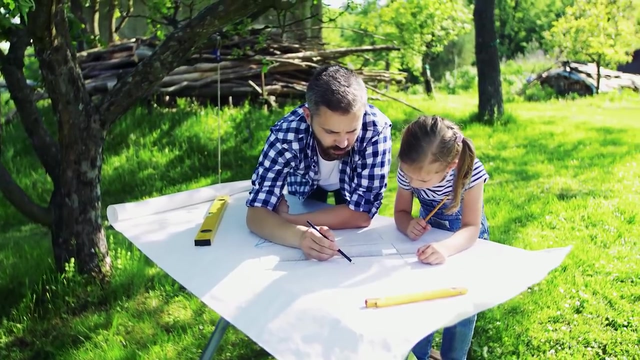 instead of using plastic bags for your lunch items, try using containers that can be washed and reused again. Reusing is finding a new way to use trash So that you don't have to throw it out. For example, you could make an empty plastic milk. 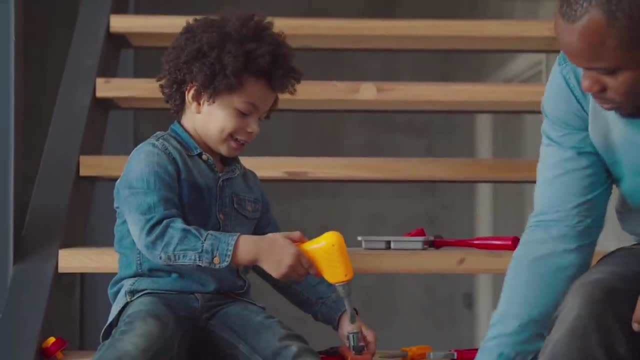 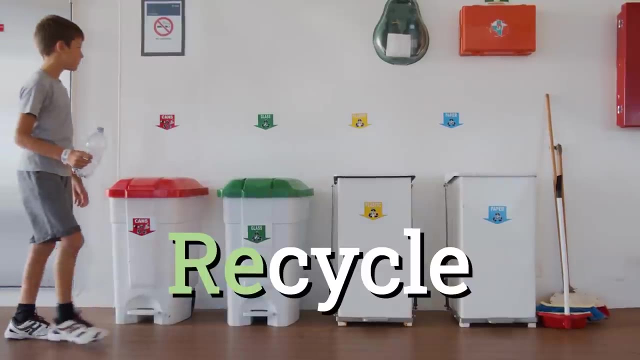 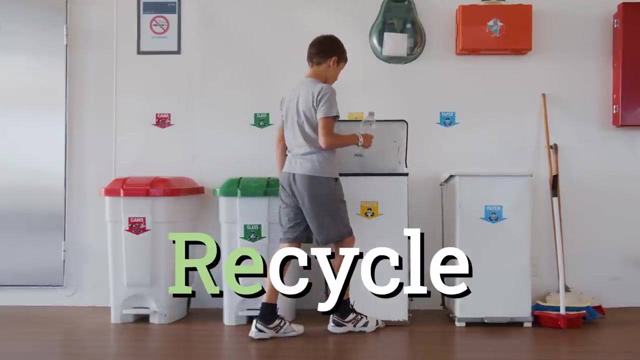 jug into a bird feeder. You can also see if something is fixable before you decide to toss it out and get a new one. Add recycling to those other two R's and you've got three great ways to help the environment and decrease the amount of trash in our landfills. The best part, It's. 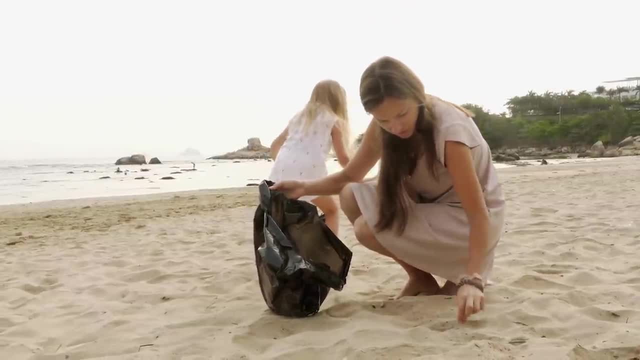 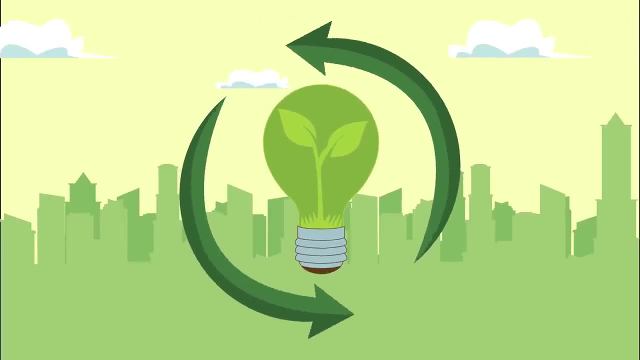 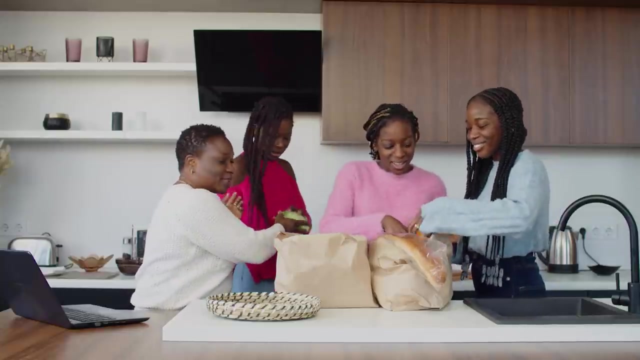 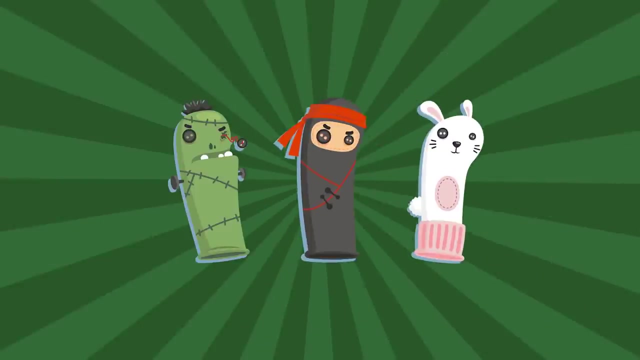 something that you can work on every day, And it can be fun. Here are some other ideas on how to reduce, reuse and recycle. Ask your parents to bring their own reusable bags to the grocery store instead of using the plastic ones. Instead of throwing out your old socks, make a sock puppet or a sock snake. Think of an. 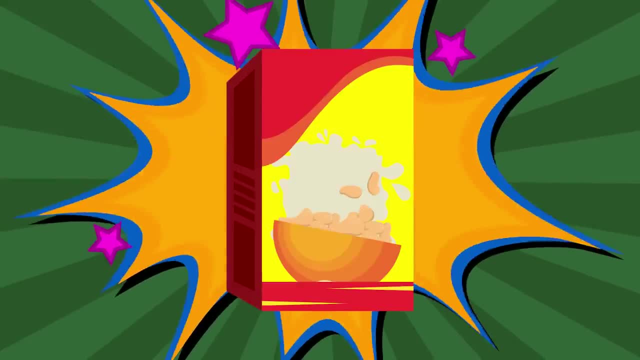 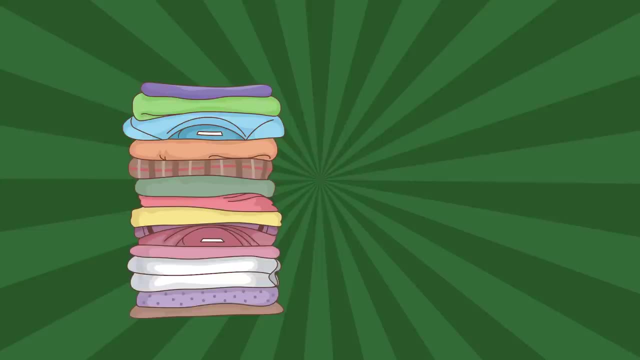 item in your house, like empty cereal boxes that can be recycled or used in an art project. Don't forget to make a sock puppet or a sock snake, Or donate your old clothes that don't fit anymore. You could give them to a friend. 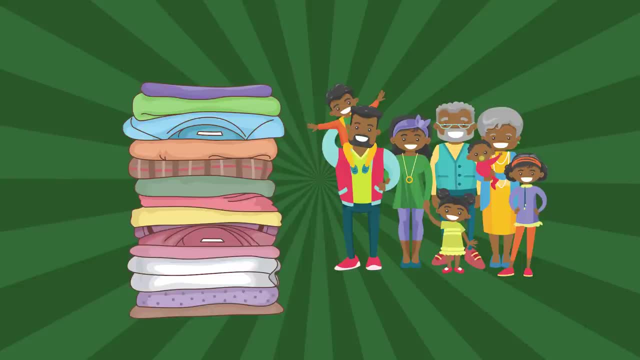 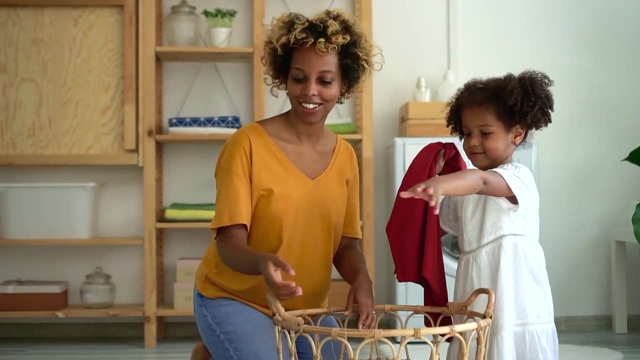 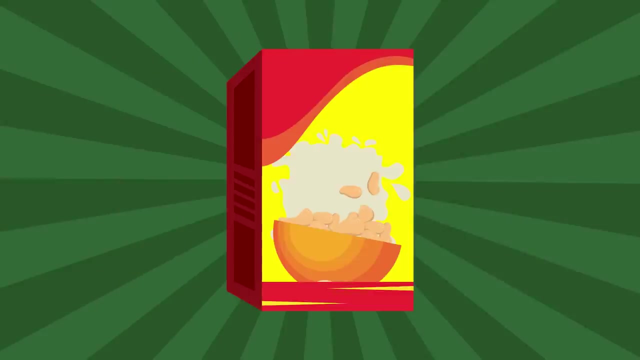 a cousin or another family member, Or take them to a place that accepts clothing donations near you. Don't forget to ask your parents for help. There are a lot of things that can be recycled: Tin cans, cereal boxes, glass jars, newspapers and mailers. 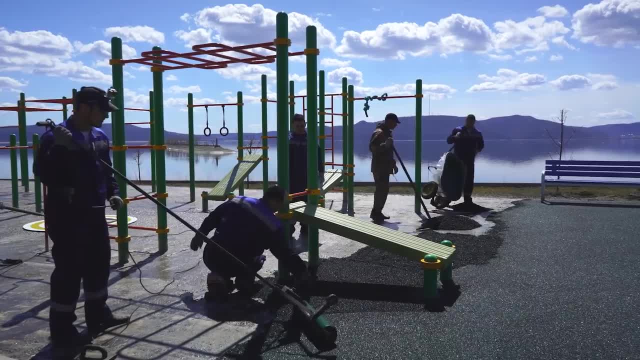 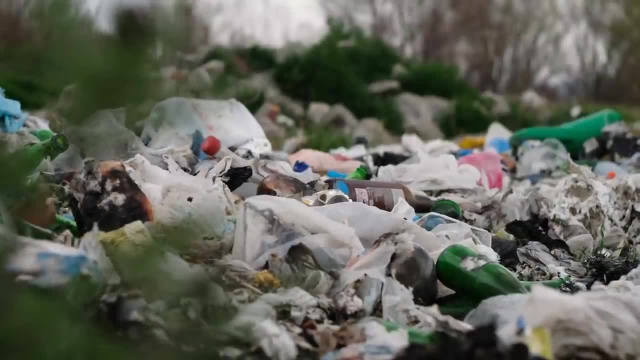 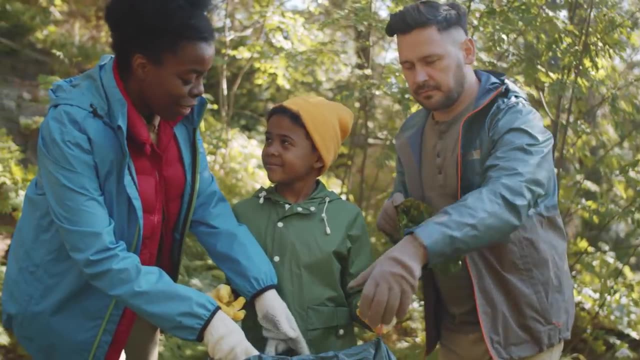 Even used car tires can be recycled into rubber mulch for your school playground, But there are also some things that cannot be recycled, So it's important to know if something can or cannot be recycled before you put them into the recycling bin. Even if you haven't recycled before, you can begin today. Get a clean garbage can or box.